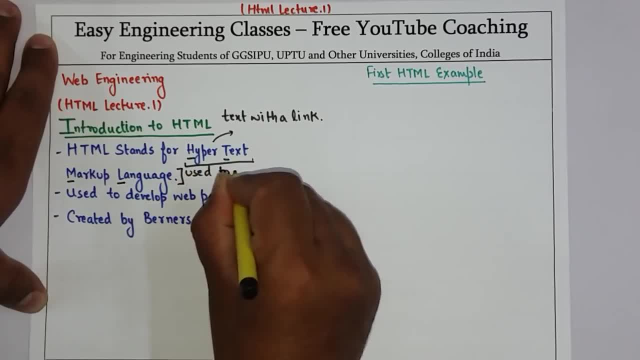 So this markup language is used to make text more interactive and dynamic. So let us see how to use Markup Language. Wait a little bit. Let's see how HTML and JavaScriptbolt is used, usually to mark blocks, So this markup language is used to make text more interactive and dynamic. 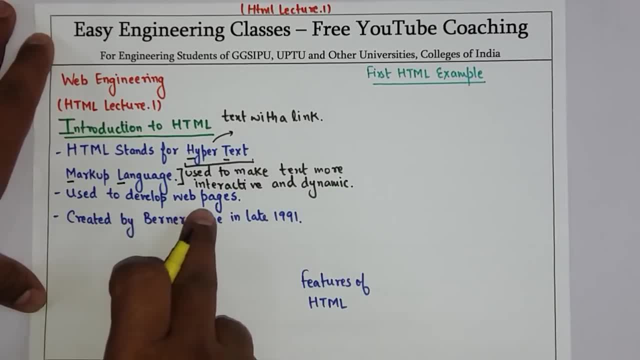 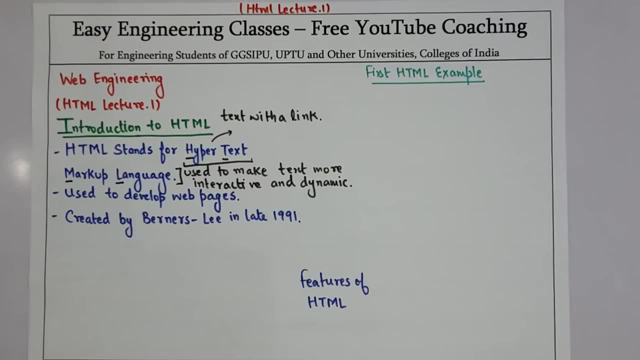 HTML is used to develop web pages. It is actually the web site web pesarivate file. It is actually the very basic language that is used to develop web pages website and it is created by Berners-Lee in late 1991.. 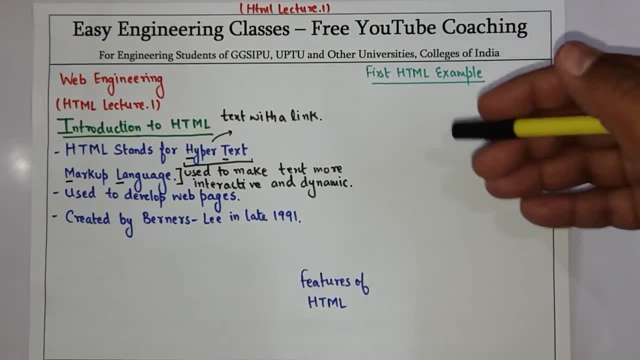 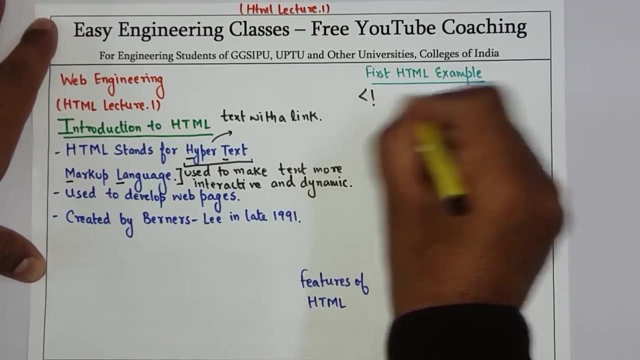 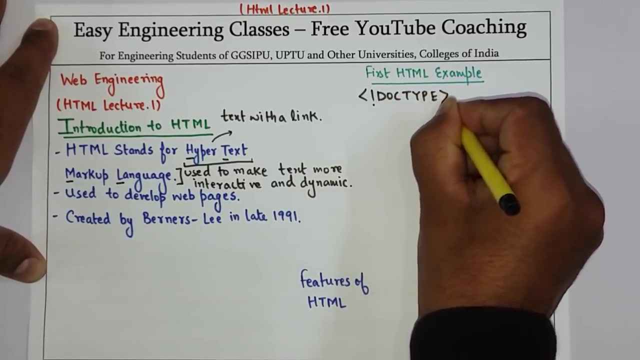 So what we are going to do in this lecture is we will see basic example of HTML and then the features of HTML. So the first example of HTML is like now. this is not necessary to write the doc type tag here, but since this is the first lecture, I am going to explain each of the tag. 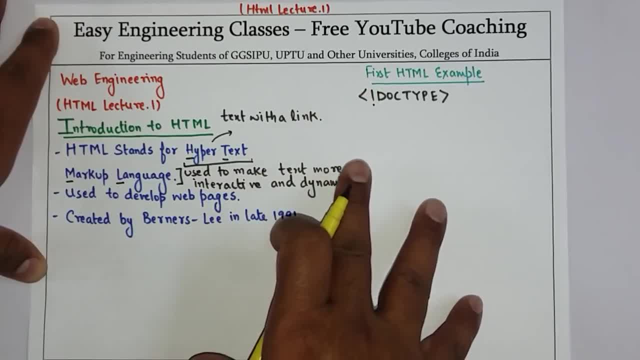 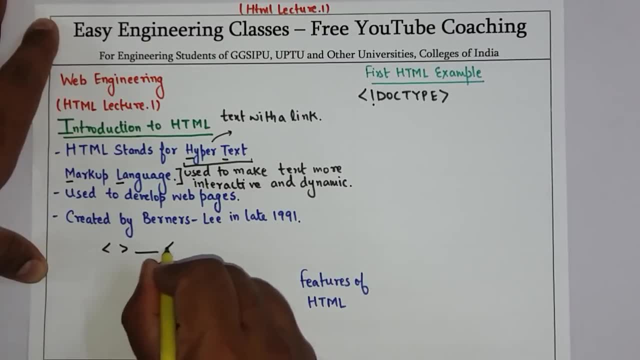 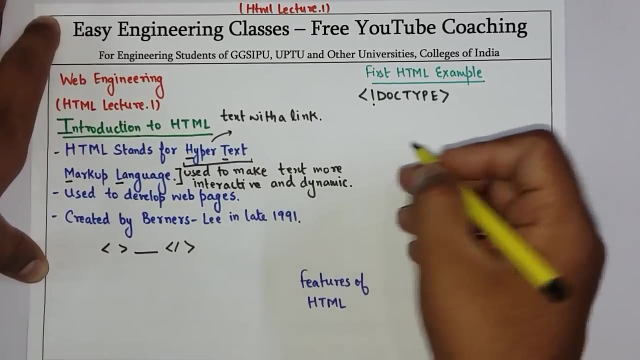 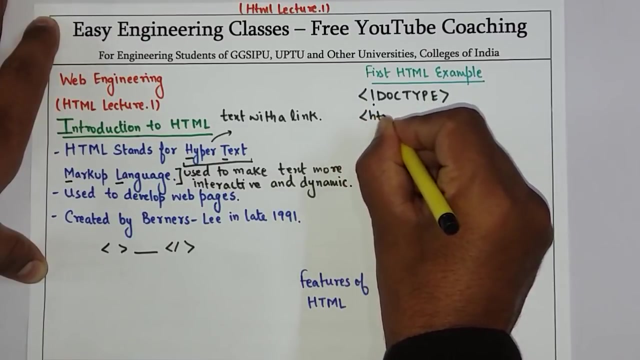 HTML is written in the form of tags. there are opening tags in which you write some content, then there are closing tags, and each tag has its own meaning or its own function. So the doc type is written To start HTML. The first tag you write is HTML. 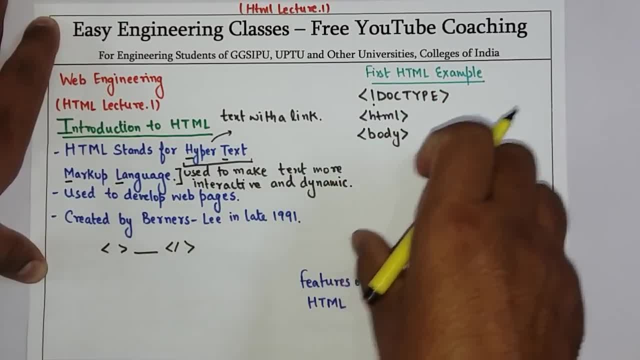 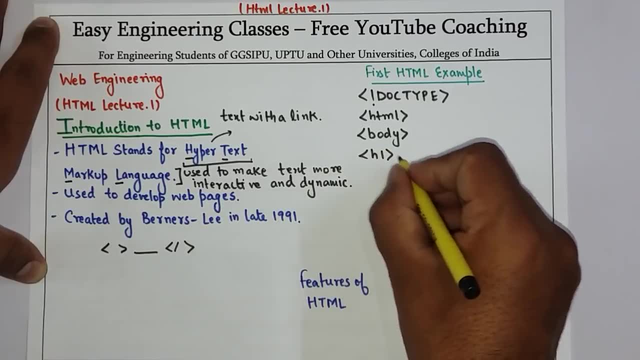 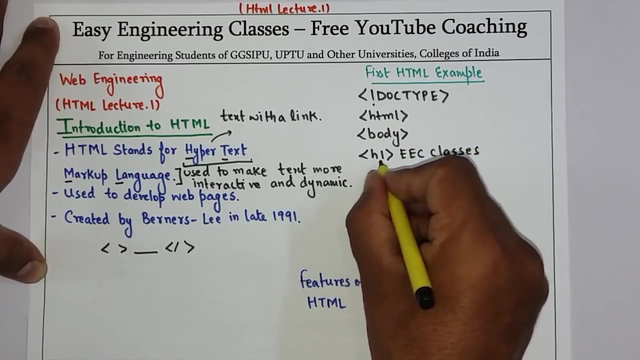 Then we have body. The main content of the web page goes inside the body. In this you can have different tags, like h1.. This is the heading tag. Now see, as I started the h1 tag here, to close this tag, we will write: slash h1.. 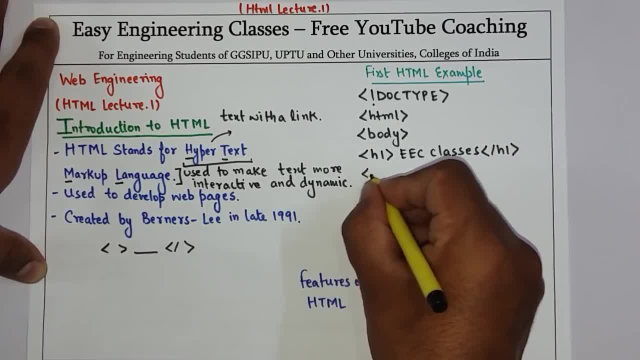 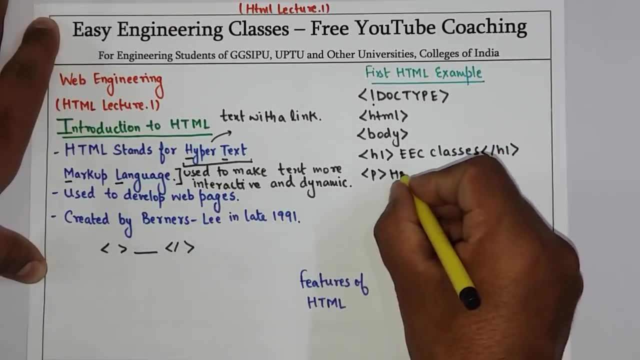 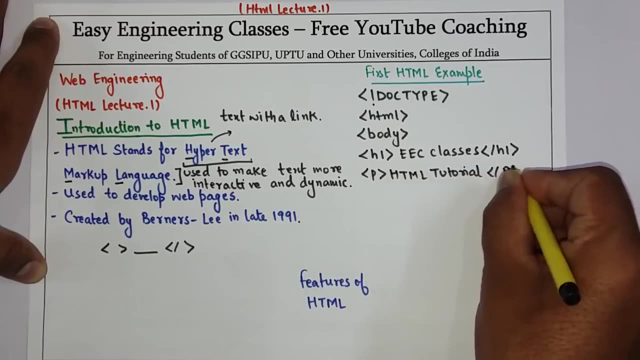 To close this tag, we will write slash h1.. After that, if you want to write in the form of paragraph, then there is a paragraph tag. For example, I wrote p, so p is for paragraph. Here we can write anything. html tutorial. then we closed the p tag. now h1 tag is closed. 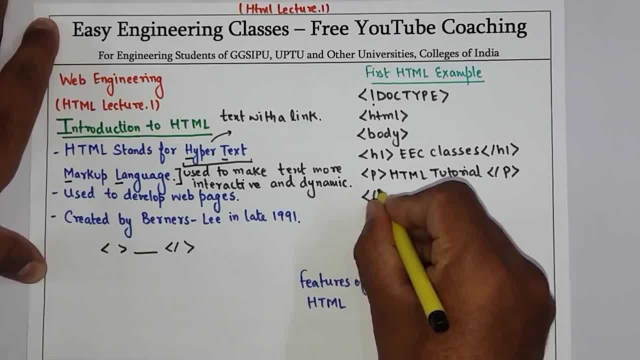 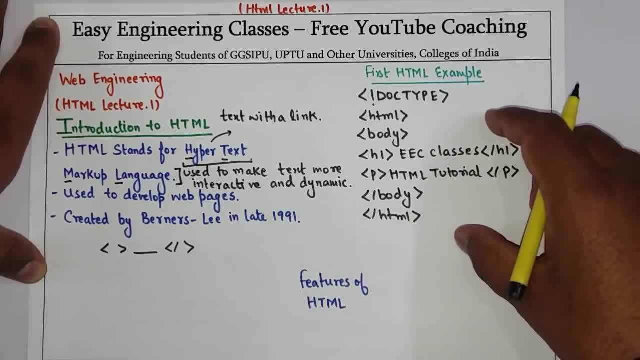 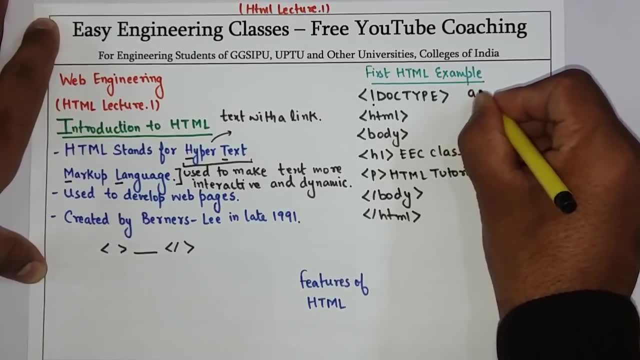 So we will close the html. So now you see what it does here. This is the html tag, So this is a basic html example. You can write this whole code in the notepad and can save it by using any name. You can give HTML or HTML extension. 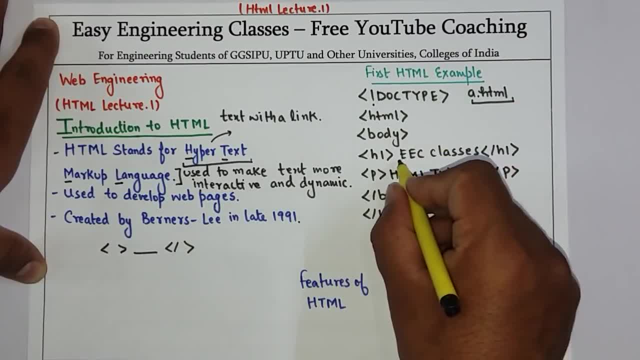 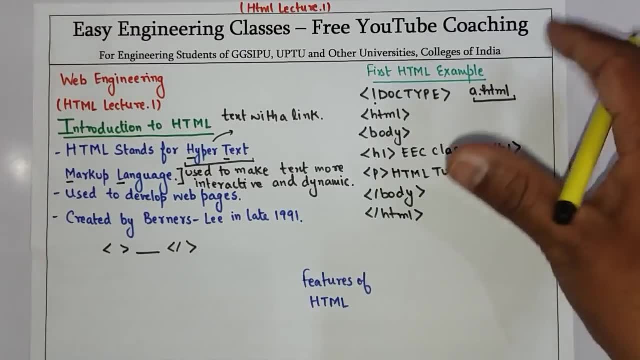 And if you open this on any browser, you will see a web page in which you will see EEC classes in the heading and you will see HTML tutorial in the paragraph below that. So let's see the meaning of this: different tags in this example. 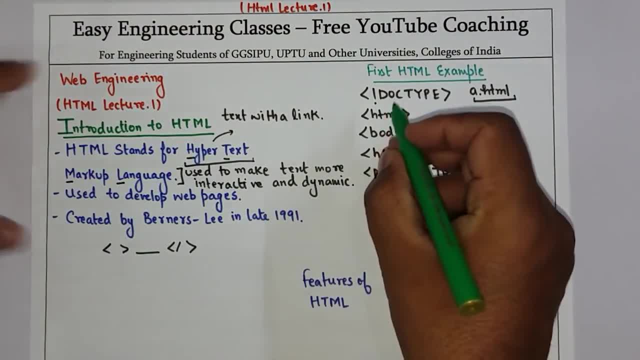 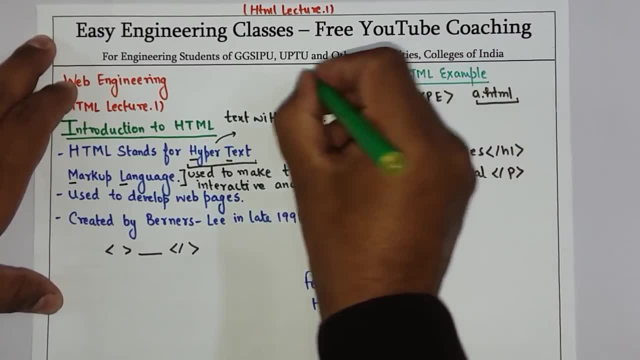 So let's see the meaning of different tags in this example. Okay, if we hit start or clinic and we come back to this chapter, then we can also see this. So the first tag here is doc type. This tag defines the document type. 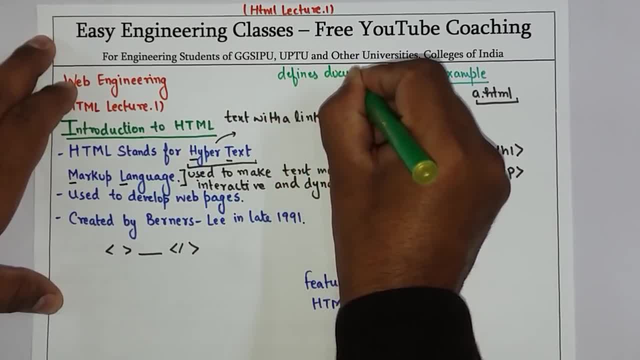 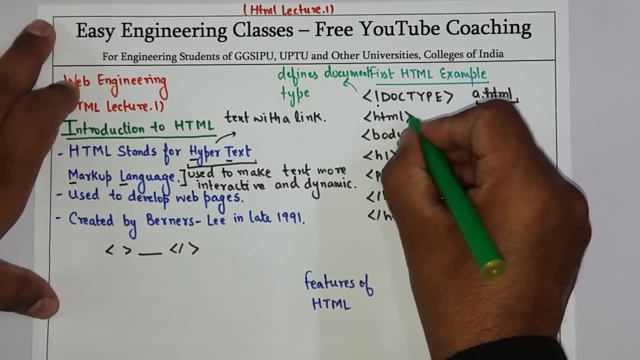 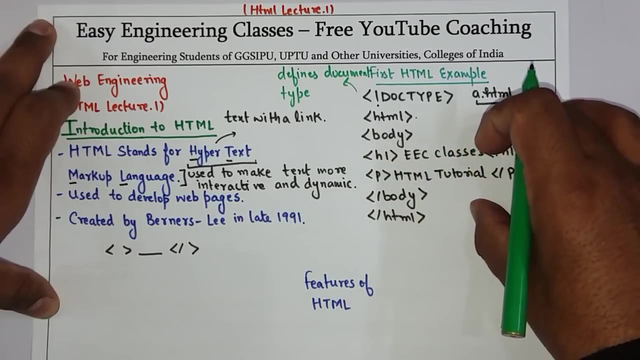 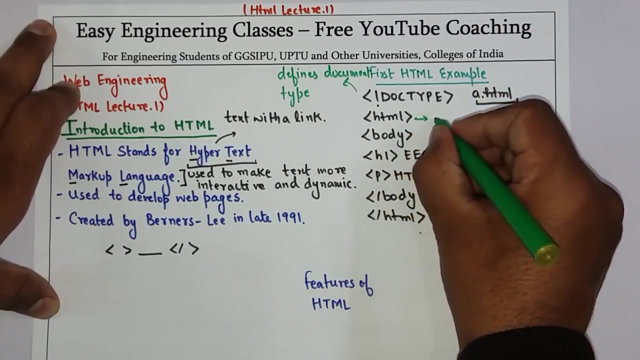 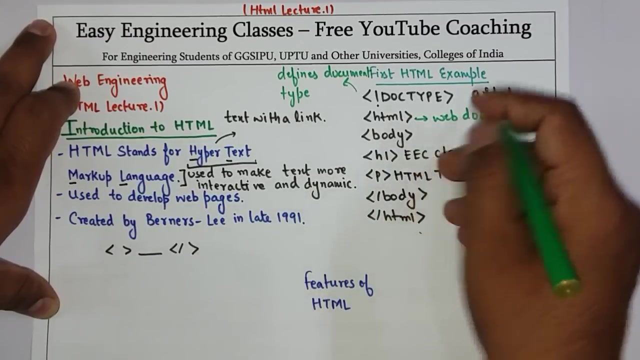 It basically defines the document type, Then the content between HTML and HTML closing tag. the content describes the web page or the web document. So the content between HTML and HTML closing describes web document. The content between body tags describes the content of the web document or the content. 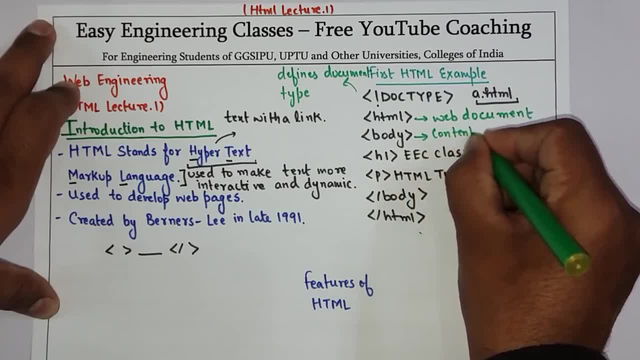 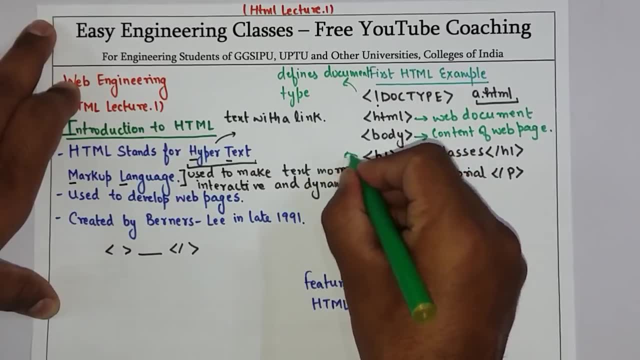 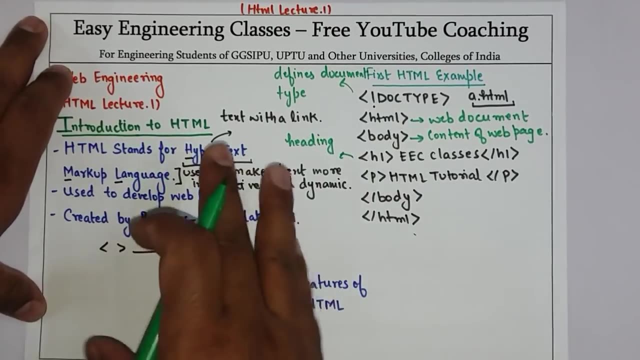 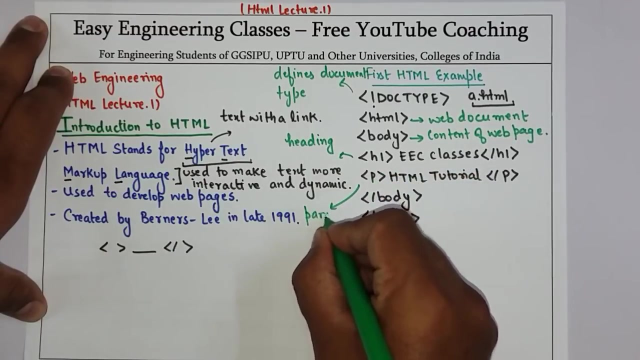 of the web page. So it is the content of web page. Now, h1 is simply the content, the heading tag. there are different types of heading tags, from h1 to h6. the main difference is in their sizes. p is for paragraph and these are the closing tags for the corresponding. 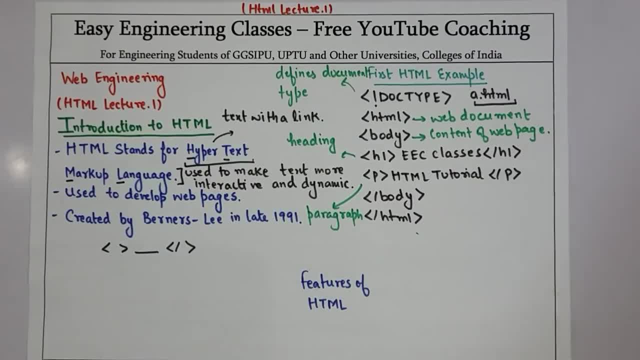 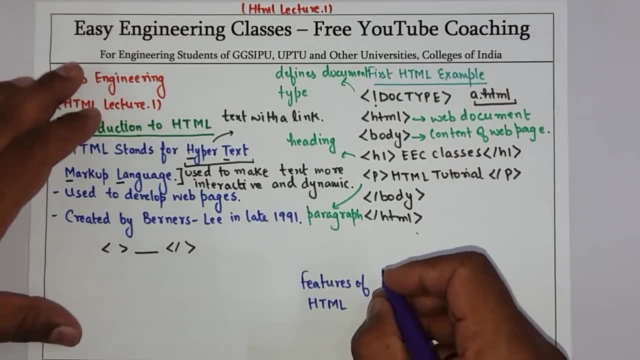 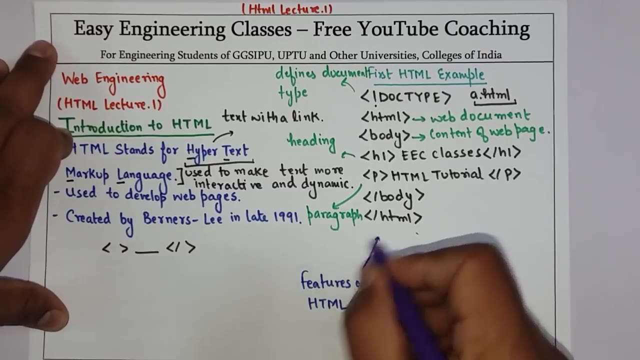 opening html tags. so this is the first example of html. now there are certain features of html which you need to know because in some, because in the theory exam sometimes, the question is: explain the features of html. so the first feature of html is: it is a simple and easy language, as you can see.